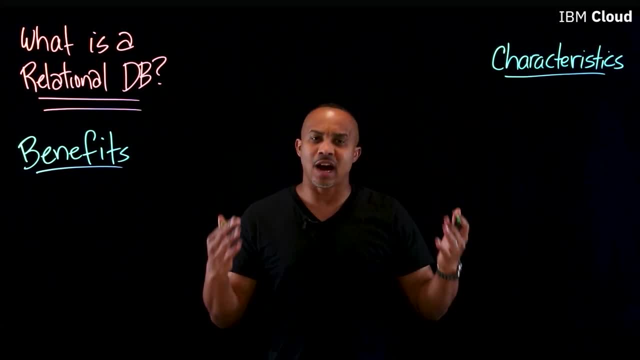 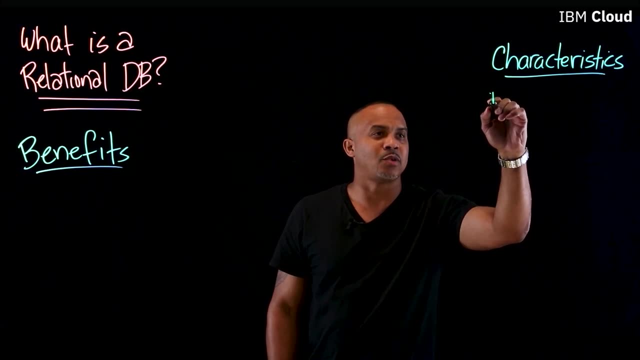 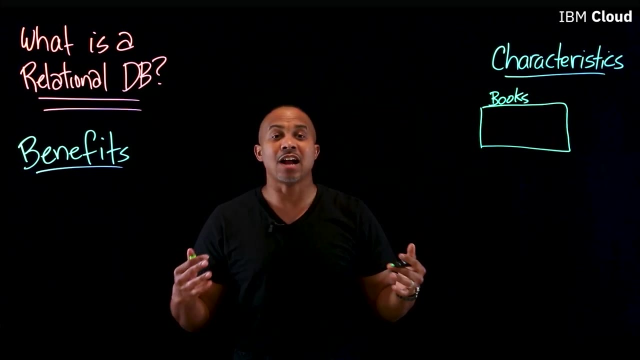 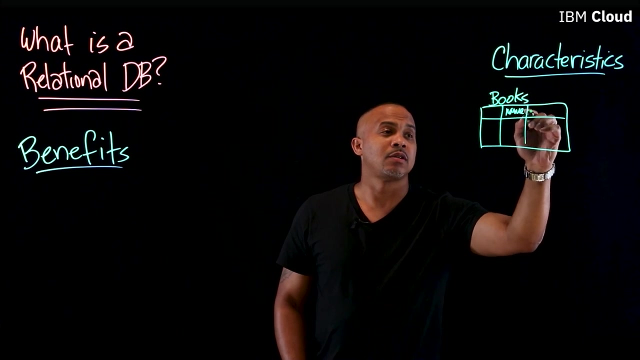 which represents particular items or nouns or particular entities of your particular system that you want to actually prototype. So let's say I have a bunch of books. Now this is going to be a table. It accomplishes the attributes of these books by having columns, And columns will be things like name, date- okay, maybe author. 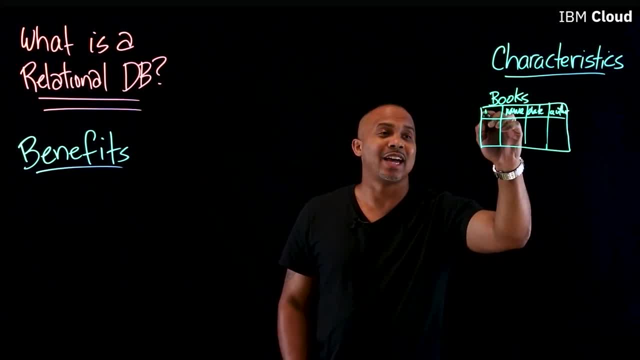 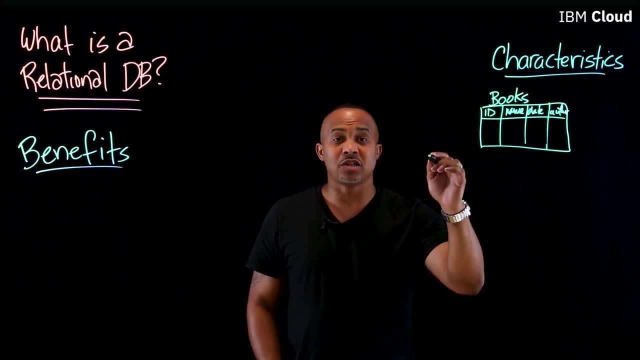 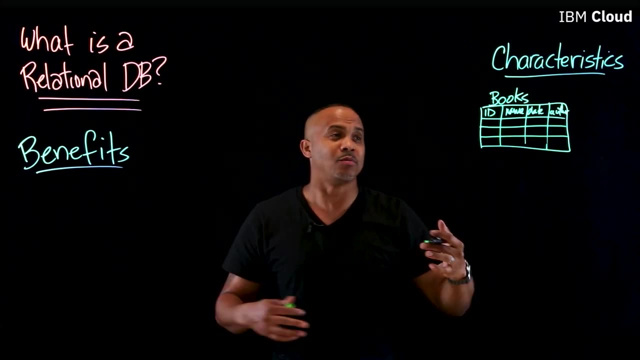 Of course, got to have an author for a book And every table is going to have an ID field, some way to uniquely identify it. Each row of this database table represents an actual record or an item, a type of book. That's how it really fulfills that ability to hold the database system there. 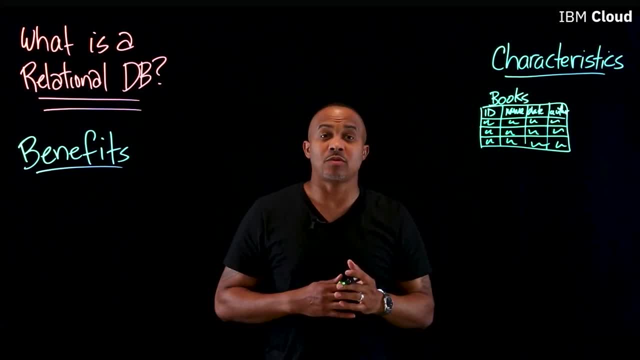 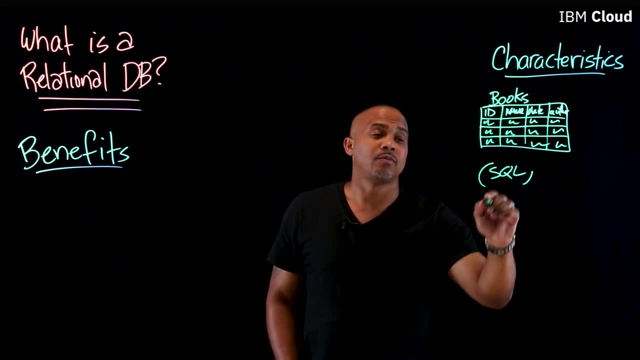 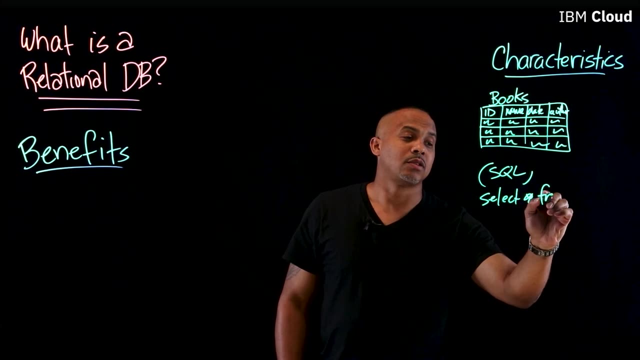 And then, as you, the way that you kind of query out this particular system is through what we call a SQL, a Structured Query Language, And it's a particular system. you can say: select all the books and give me all this data out for me to use. 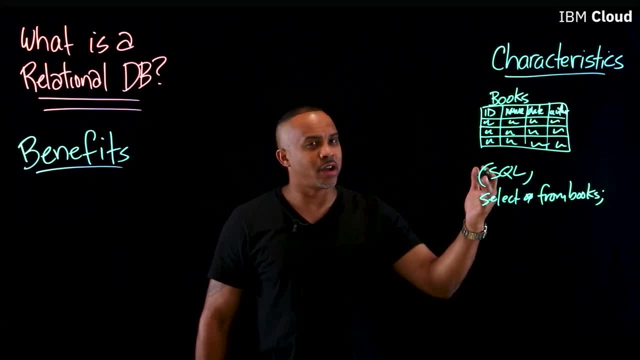 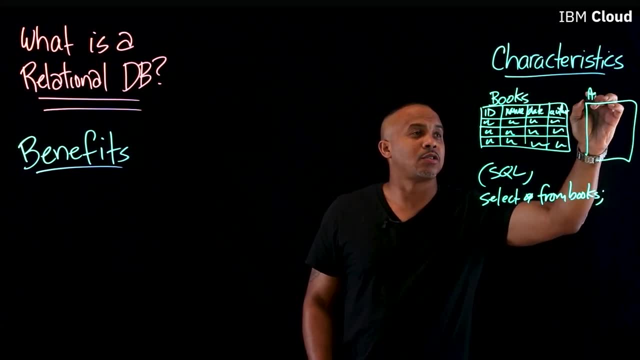 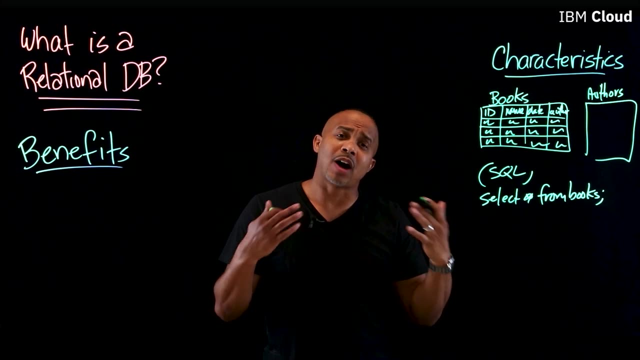 Now we have one particular item here: books. but where it really comes, you really see the power of a relational database. Let's say, now I want to show the authors And the way that relational databases can really provide the structure of relating these. 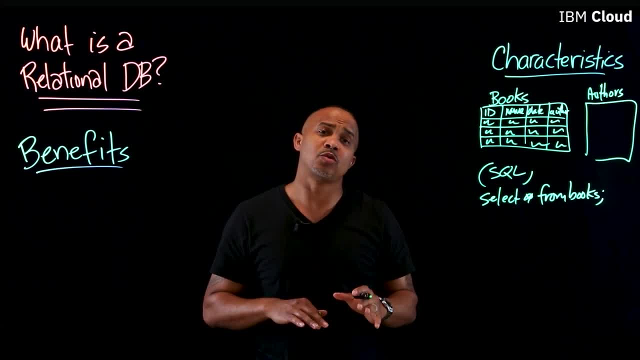 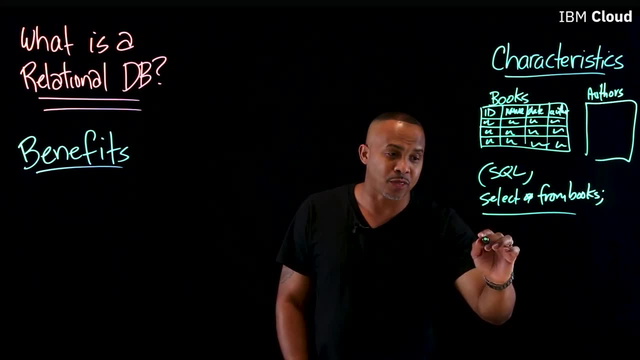 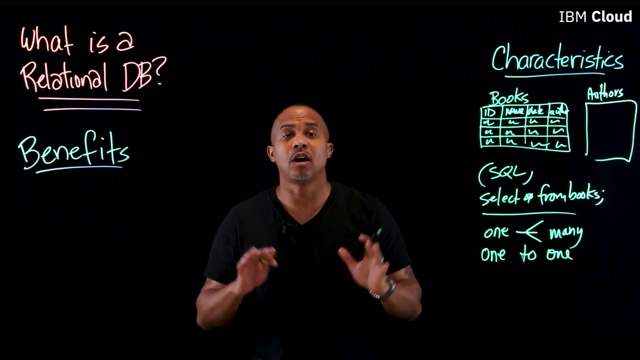 two entities together is by describing them through a particular entity or relationships. You have one that you'll hear about, where books can have multiple authors, so maybe a one, two, many. You can have a one, Two, One, Maybe just a couple of relationships you can kind of mirror within the database system. 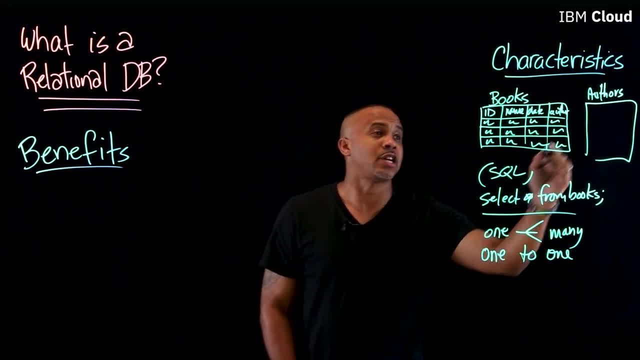 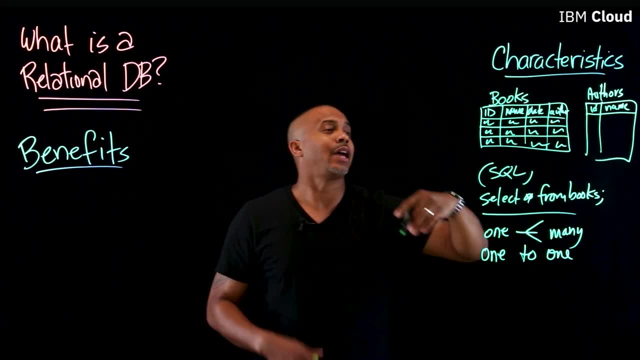 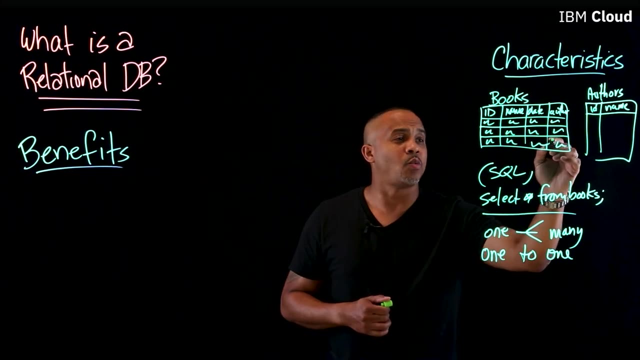 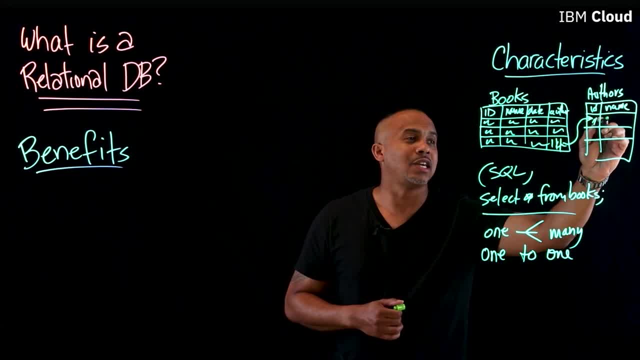 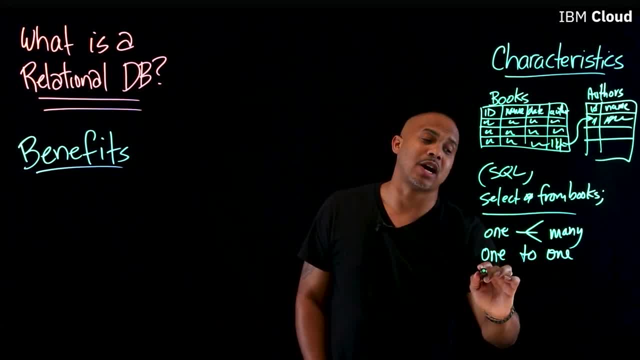 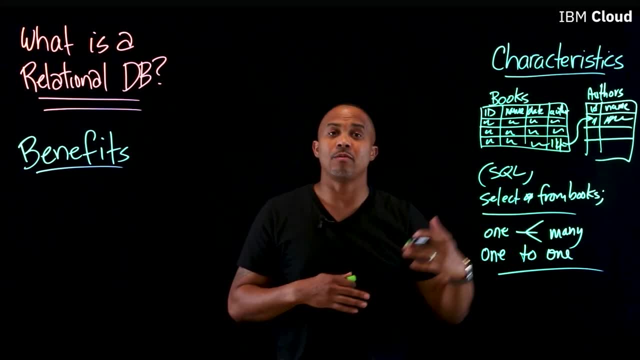 And of course that'll be a name there. So when I do my query, the next query I do, I can reference both these tables and say, hey, give me all the books and give me more of the author information from this table. 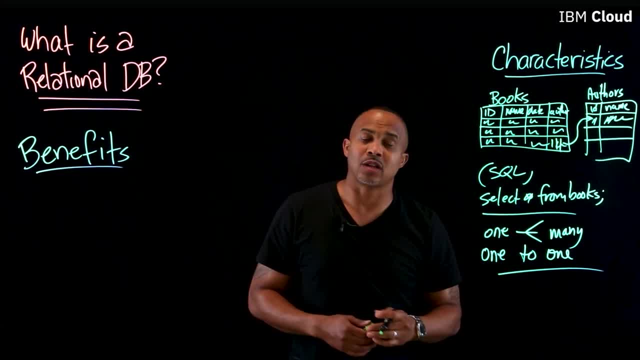 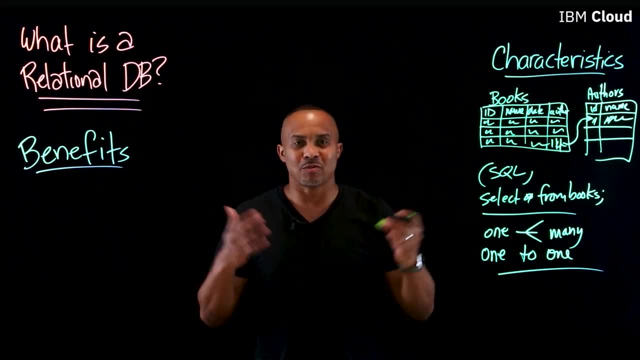 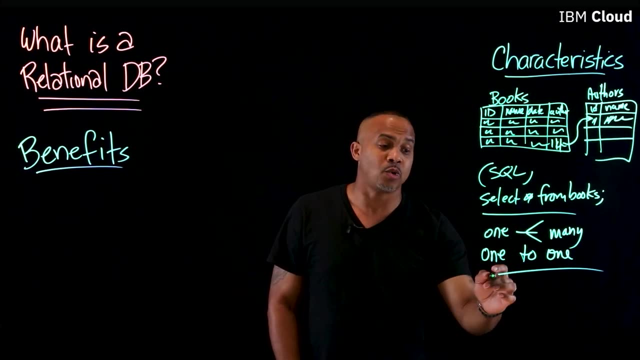 using this foreign key to describe that particular structure there And you can imagine you'll be running a lot of these queries, a lot, and there are some benefits or some things that are provided to help with those, to speed up these queries and make them operate as efficiently as possible. 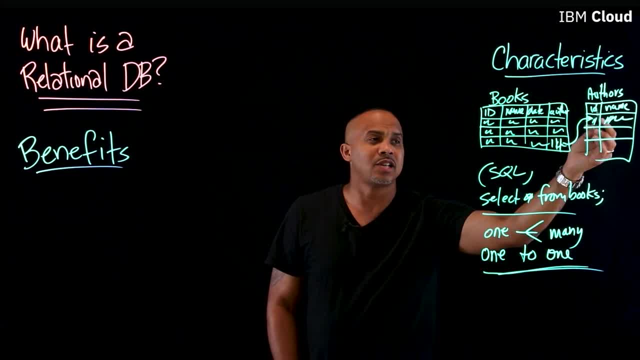 You have the database will provide ways that you can kind of set an index. Let's say that I'm often querying and always trying to pull out by name or by date. I can set an index on this particular column which will automatically index all the values. 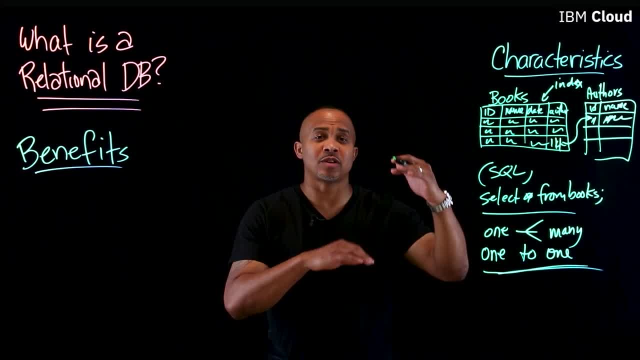 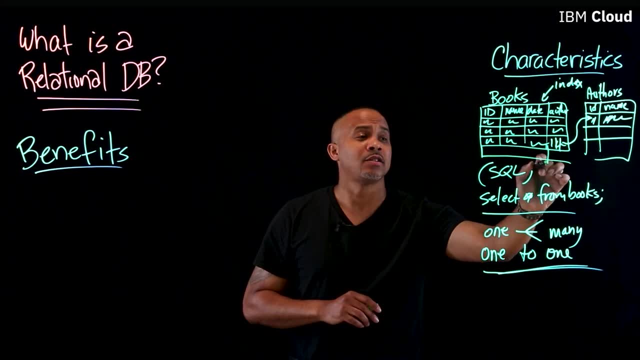 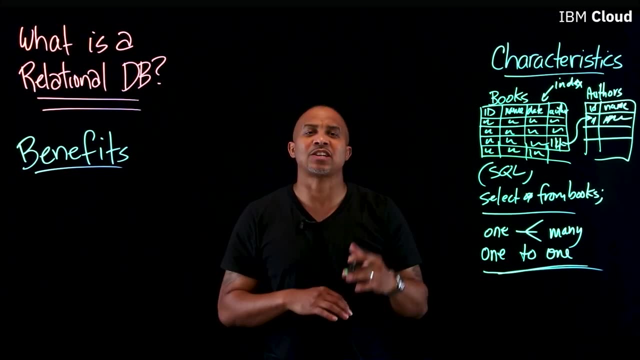 So the next time you run this query, it's going to pull from what we like to call this cache of all the values. Most importantly, every time new rows are added, records are added to this particular table, the index keeps building this recent- I like to say- cache of all these values. 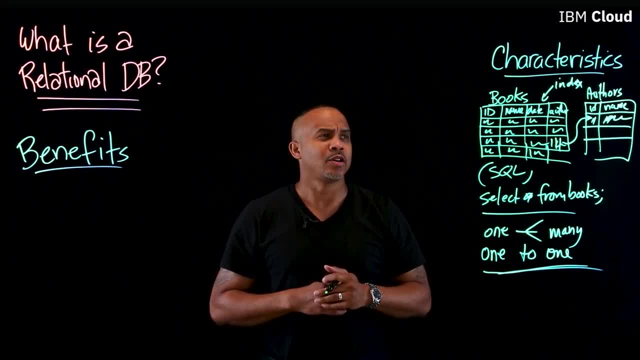 So it's always keeping up to date to work there. So this is all the characteristics of what you kind of have to model out your particular application that you want to build And describe how the entities are related to each other. Now let's switch over here to some of the benefits that you're going to get out of the. 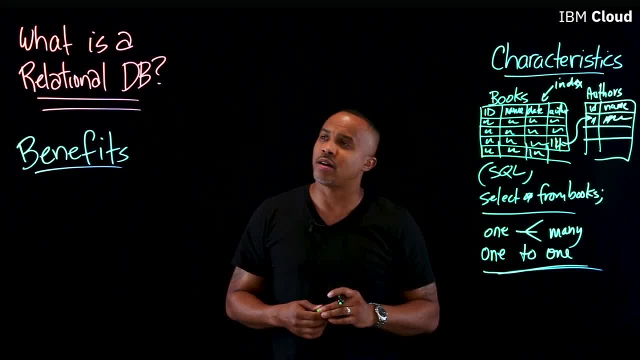 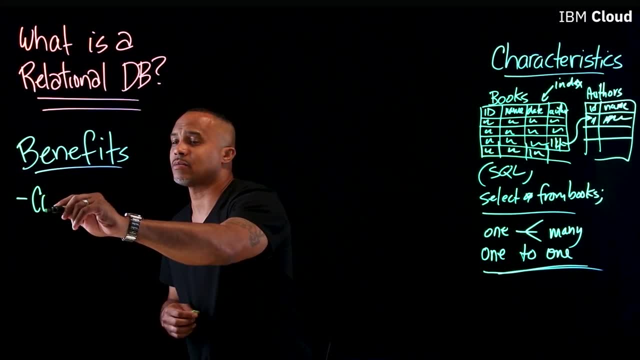 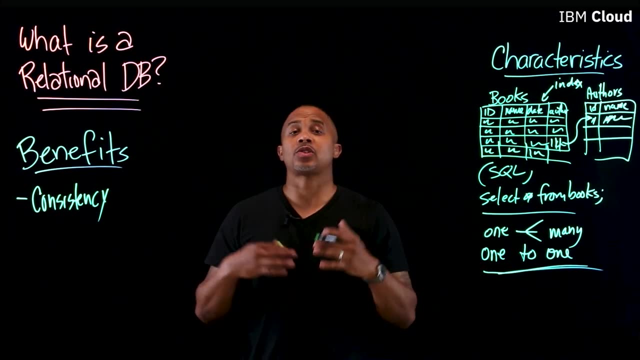 box with a relational database that you want to use. The first we'll talk about is actual: the consistency. Now, this is useful because, let's say, there is some point where I want to run multiple of these transactions. Let's say I'm modeling. 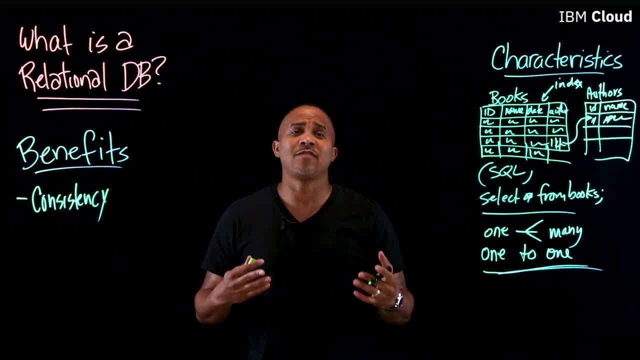 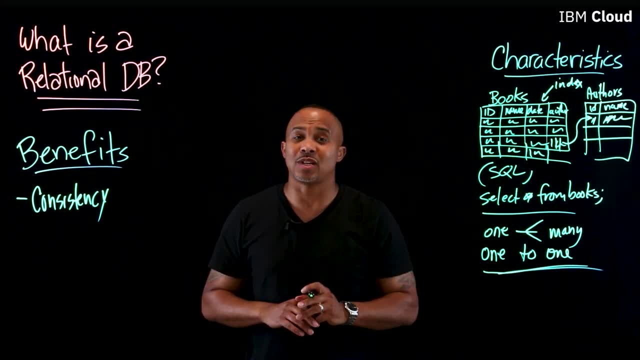 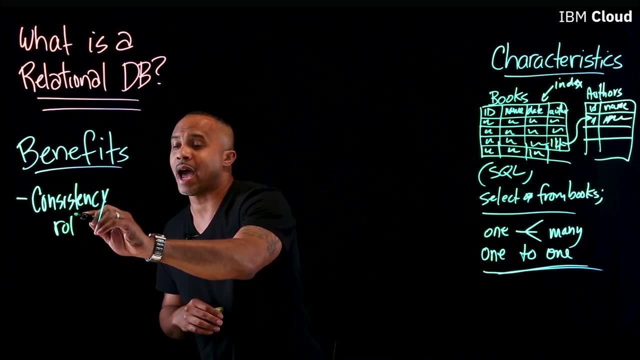 Let's say I'm running an inventory system for an e-commerce application and I have the need to write several queries in a row that may manage a couple of different subsystems, But if one of those queries fails, I want the option to be able to roll back the whole. 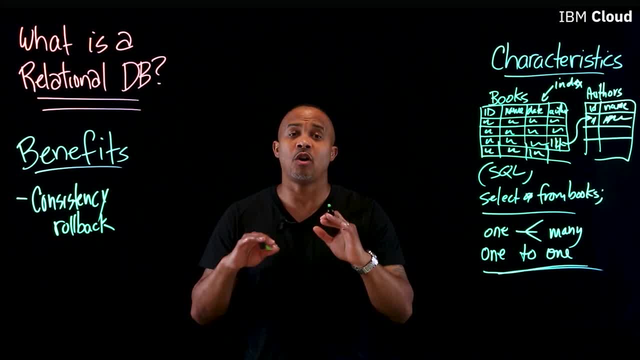 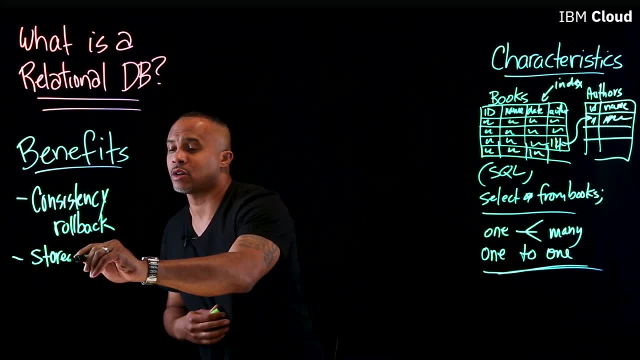 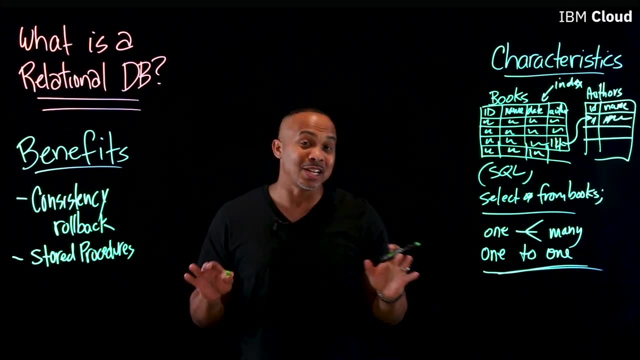 set of all those queries just to make sure that my data always maintains some consistency there. The second is the option to do this. The third is the option to do stored procedures. Sounds like a very complicated word there, but think of stored procedures as the ability. 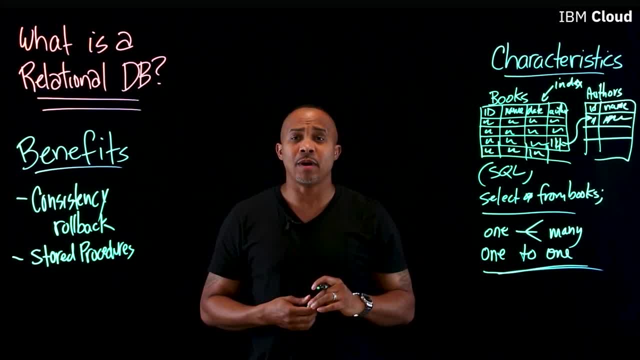 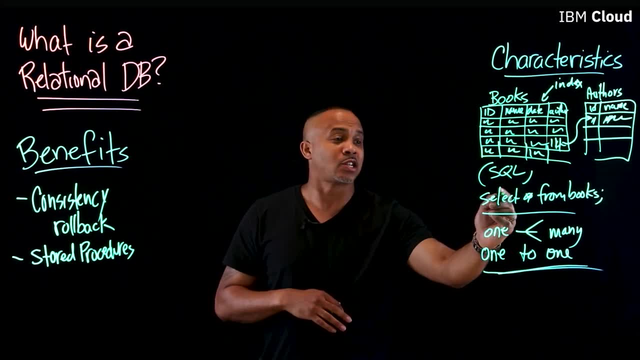 to write multiple blocks or functions of code. Or if there are a certain amount of queries that I continue to always run, I can kind of model these so it takes me less code to write that particular, to access that same functionality with less SQL code. 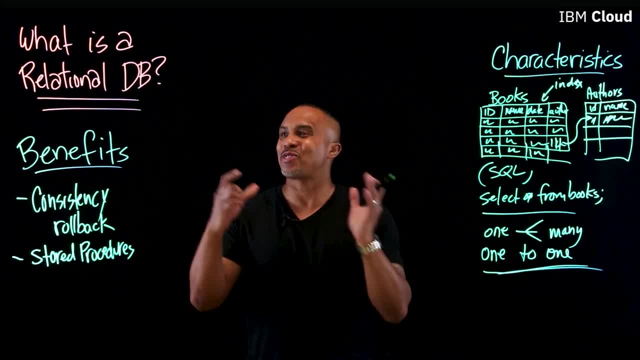 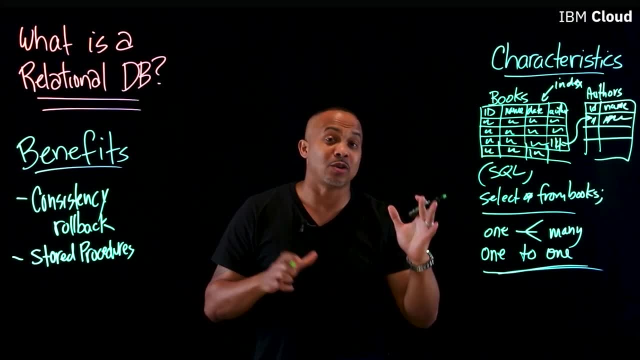 And as you start to get into more SQL applications, you're going to see that there's a lot of different ways to do this. Writing with relational databases. you'll see queries can get pretty big. Another way you can do this as well is another topic called views here. 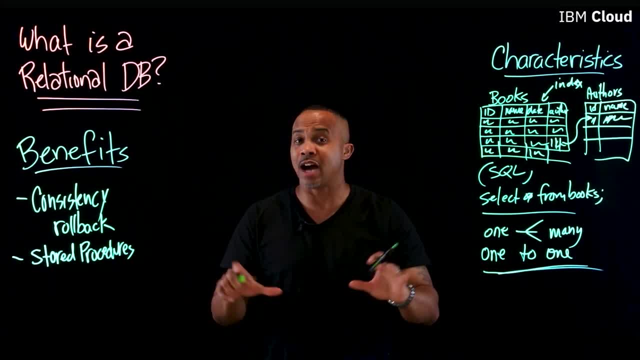 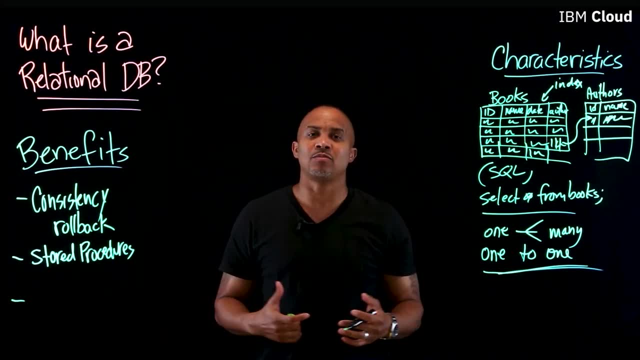 Definitely want to introduce some of these keywords. As you do your deeper dive, you're able to see a lot of these and it be familiar to you. And the last one is a mechanism to handle locking in the database and concurrency. Why, Why? 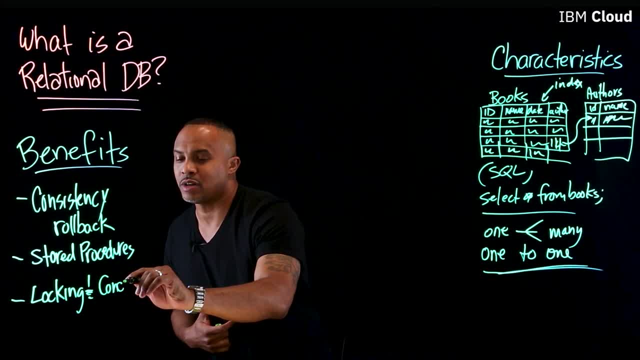 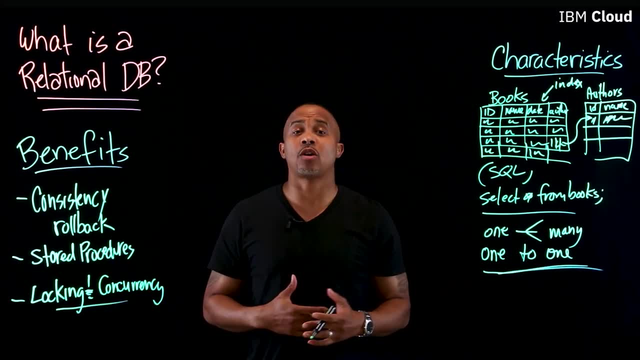 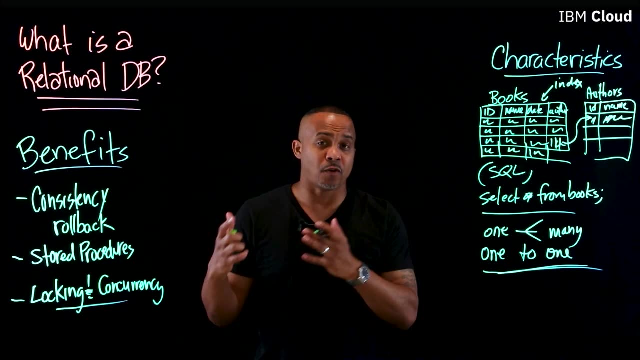 Why, Why, Why is that important? Well, at some point multiple users are going to want to use the database, maybe at the same time, Maybe two applications are going to be adding in books, And if the first application is making a particular insert into this table you're going to want 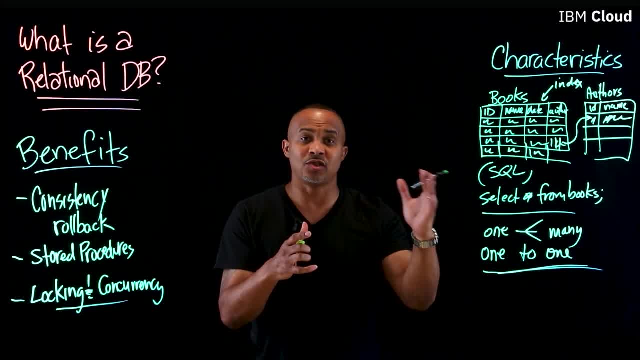 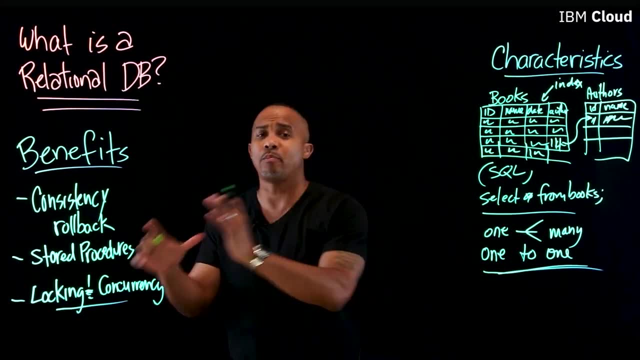 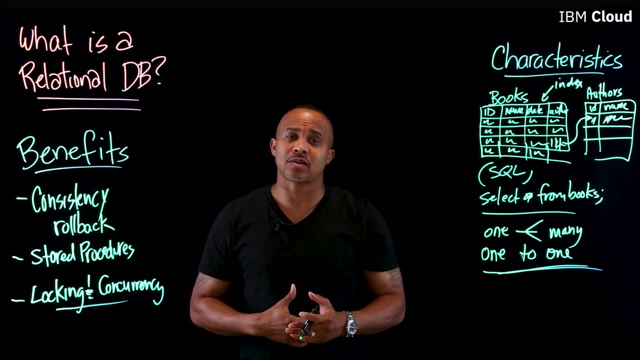 to make sure that the database is locked until that write is done. And then the second application has this ability to go ahead and make its insert As well. So these are all built into a lot of the relational databases that you use. A lot of these benefits will be provided for you out of the box. 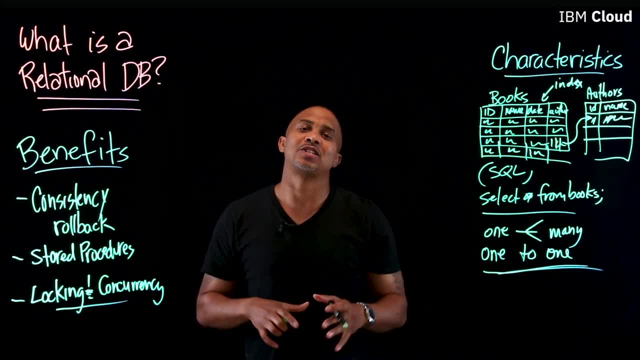 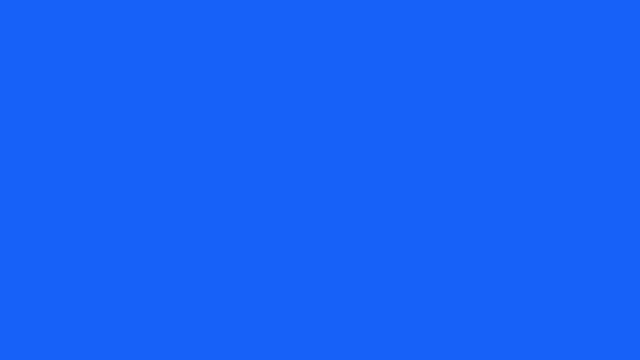 Not necessarily something you'll have to write in code, but just know that you'll have this at top of mind when you are kind of selecting to use a relational database for your next project. I hope this is good for you to understand the foundation of relational databases. 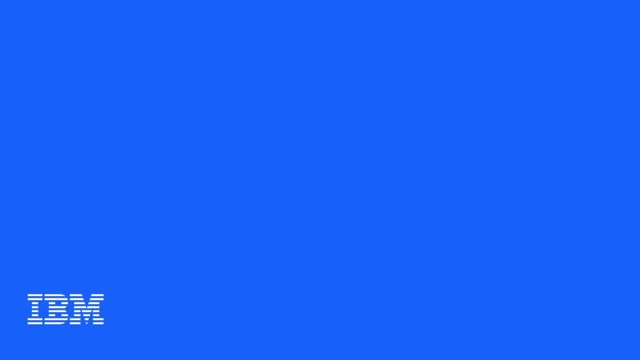 Talk to you next time. If you have questions, please reach out to me. Thank you. Please drop us a line below And if you want to see more videos like this in the future, please like and subscribe.